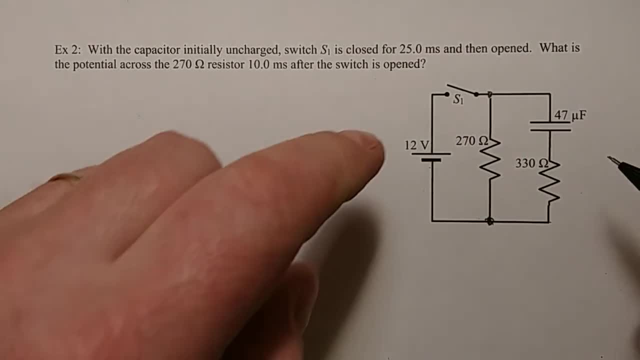 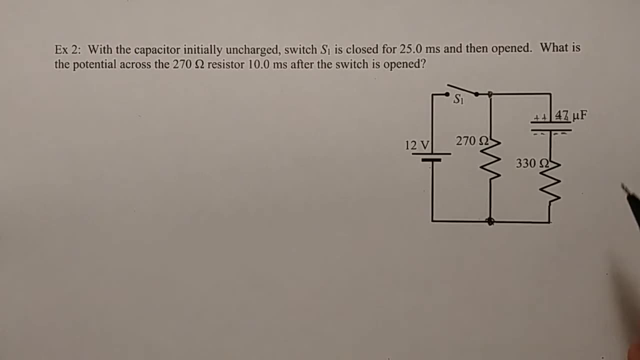 volts across it, So it doesn't make any difference. But when I open the switch again and this thing has a bunch of charges on it, those charges want to flow the other way if possible in order to discharge. And when that switch is open, 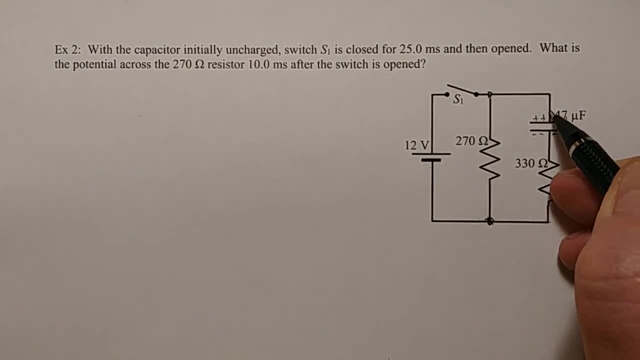 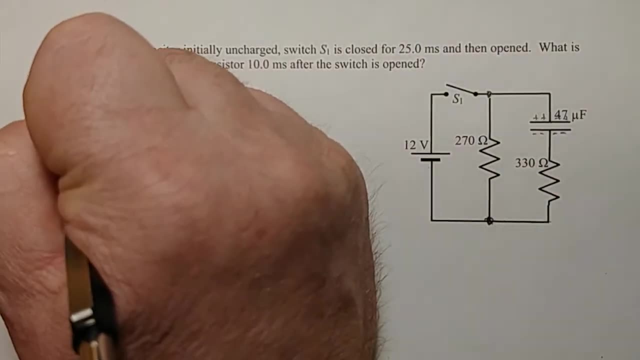 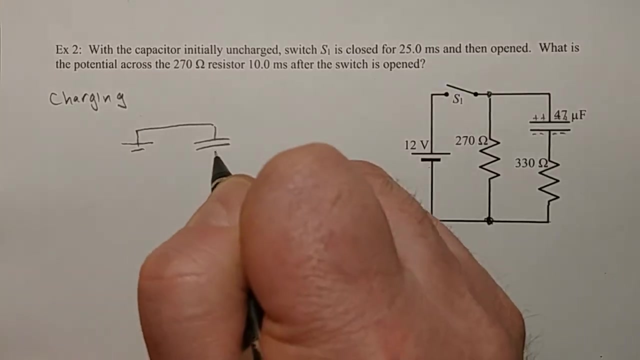 yeah, they can flow this way to discharge, So they're going to do that. So when we're charging, we have- we really just have this 12 volts, We have this and we have this and that stuff in the middle doesn't really make any difference, because this one's going to be charging up this. 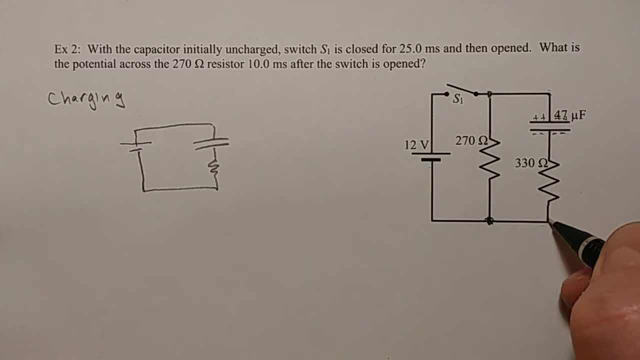 12 volts is still. this side is 12 volts compared to this. This is 12 volts potential higher than this. If you think about a Kirchhoff loop roll walk, then you go up by 12 volts, you go down by. 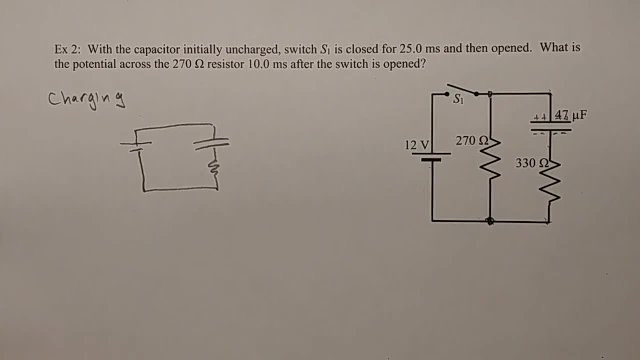 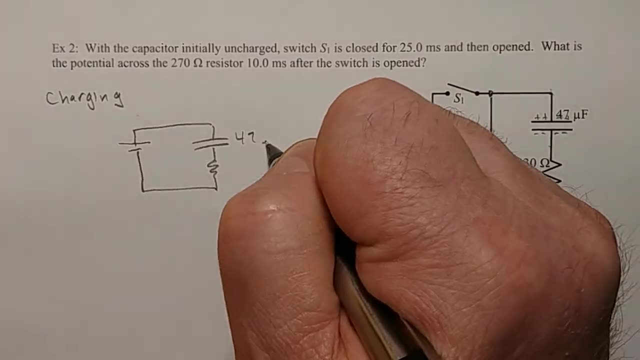 something, you go down by something and you come back to where you started, and the 270 doesn't matter. So what you have here is you just have your 47 microfarads and your 330 ohms, And so, for charging, what we're going to do is we're going to have this 12 volts compared to this. 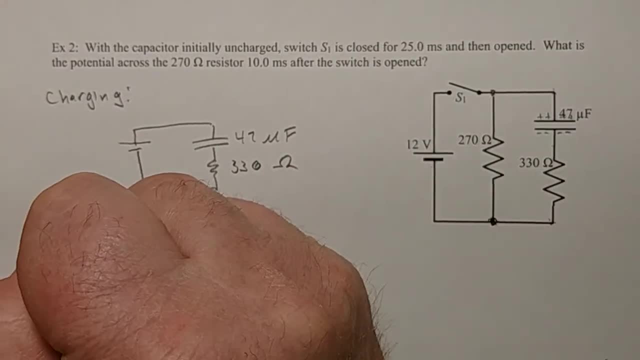 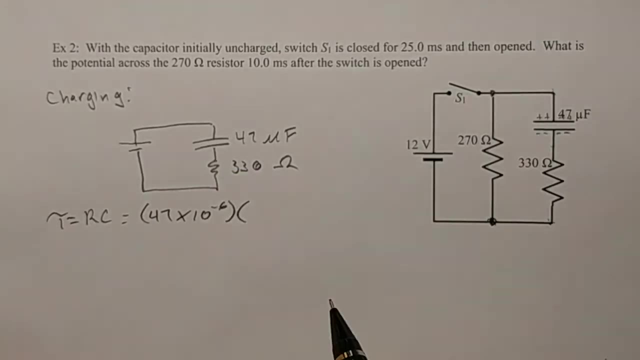 For charging. what we're going to do is we're going to have an RC. a tau which is equal to RC is going to be equal to 47 times 10, to the negative 6, multiplied by 330, which is equal to. 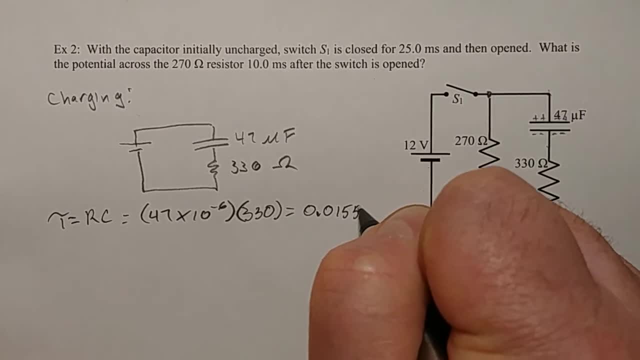 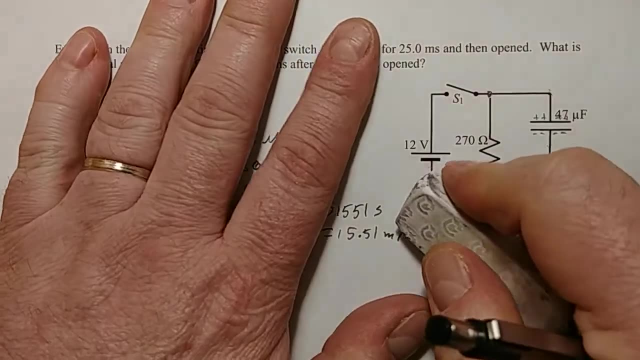 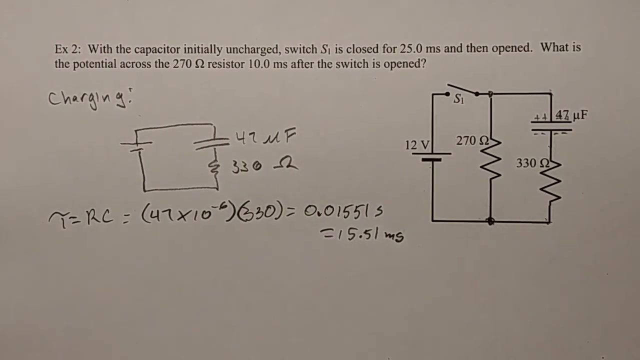 0.01551, or, if you want, 15.51 milliseconds. Whoa, there's no slash in milliseconds. Okay, So what do we want to do? We want to do. It's closed for 25 milliseconds, So. 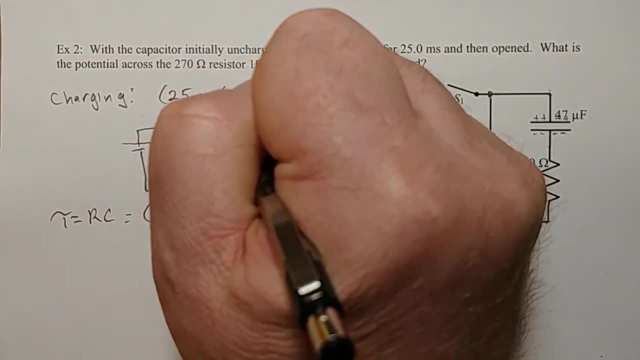 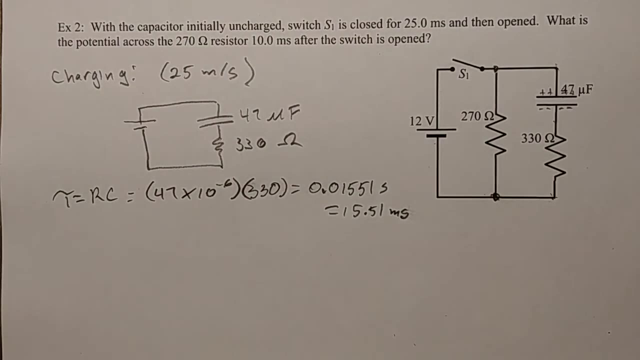 we're charging. We're charging for 25 milliseconds, Okay. So what happens is for charging, we have that formula and we can do this whole Q stuff, but I'd rather use the formula for V: V equals E times 1 minus E to the negative T over tau. Right, It's heading towards that. 12 volts. So it's equal to 12 times 1 minus E to the negative, And this is in milliseconds and that's in milliseconds And the milliseconds is going to cancel to give a pure ratio. So we can just say 25 over 15.51.. We don't need all the 10 to. 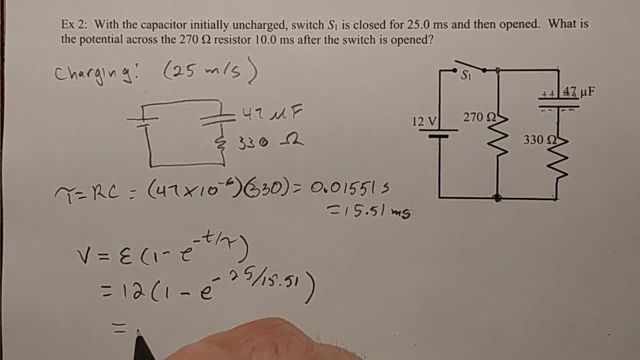 the minus stuff And if we work all that out we get 9.606 volts. So during those 25 milliseconds that this is going to cancel, So we're going to cancel, So we're going to cancel, So we're going to. 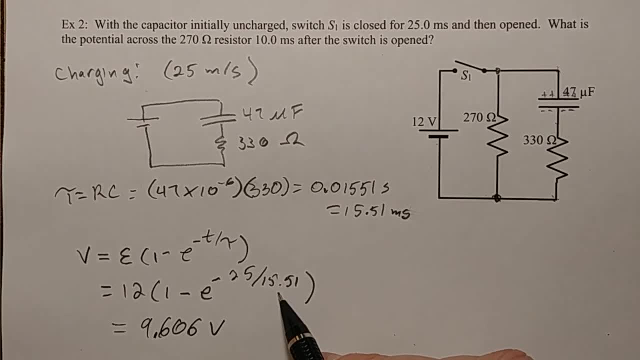 close. 25 milliseconds is more than one time constant. One time constant gets it to about 62%. So yeah, it's going to be more than 62%, It's 12, I don't know, it's like three quarters. 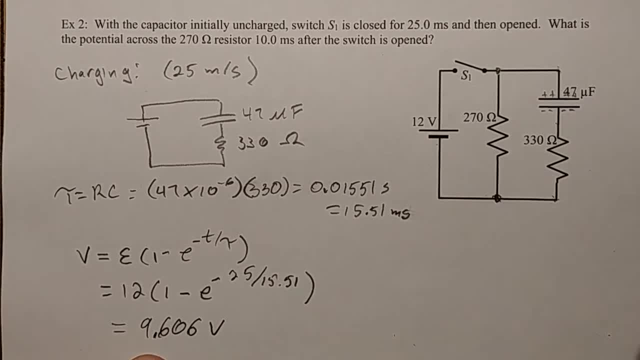 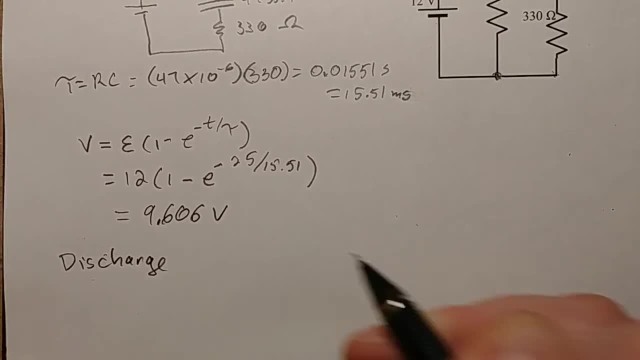 it's 80%. Anyway, it's getting it close to the voltage of the battery. But then we stop, and now we discharge. And what happens when we discharge? Well, when we discharge, we have this capacitor and the current flows through here and it goes through this resistor. 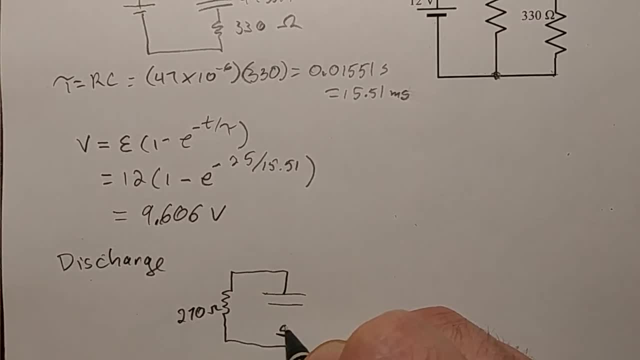 and then it goes through this resistor- Whoa, what an ugly resistor- As the charges flow this way. So to get tau, which is equal to RC, now we have to take the resistance of that whole circuit, and the current that flows through here has no node to get. 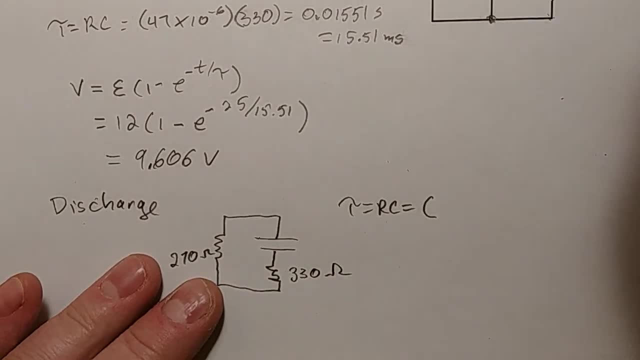 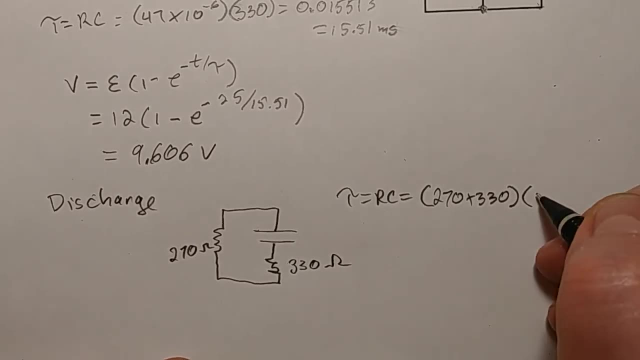 distributed, It has to go through here. So those two are in series. We just add them up multiplied by the capacitance. So we have a current that flows through here and the current that flows through here has no node to get distributed. We just add them up multiplied by the capacitance. 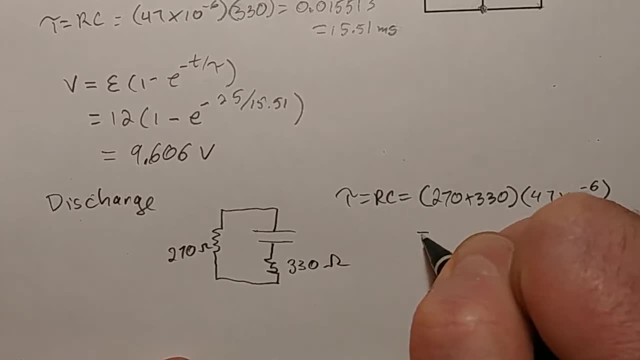 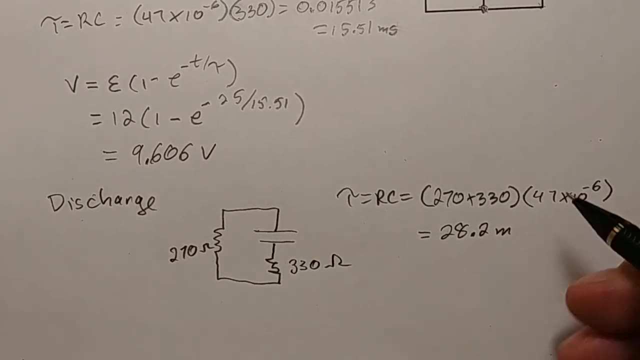 which is 47 times 10 to the negative 6.. And so that is equal to- and I'll change it to milliseconds again- 28.2 milliseconds, 28.2 times 10 to the negative 6 seconds, or 2.82 times 10 to. 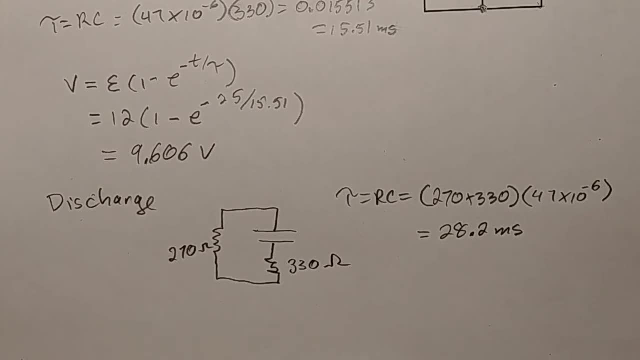 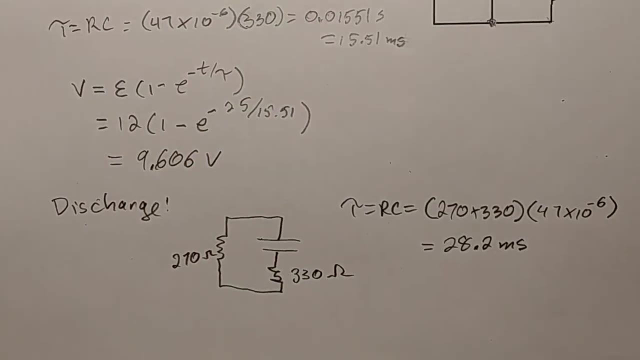 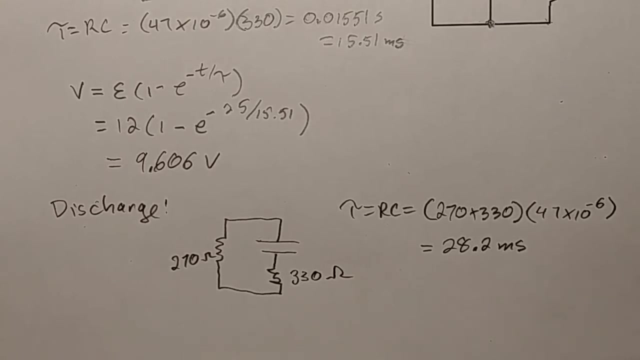 the negative 2 seconds, whatever. Okay, so that's for discharging. What do we want to do here? What is the potential across the 270 ohm resistor? 10 milliseconds? the potential across the resistor? Hmm, The potential across the resistor. Maybe we should find the current. 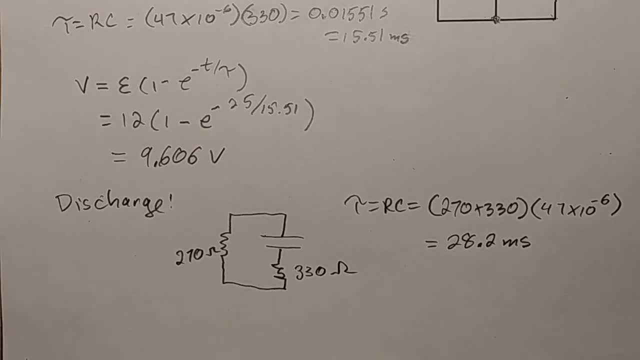 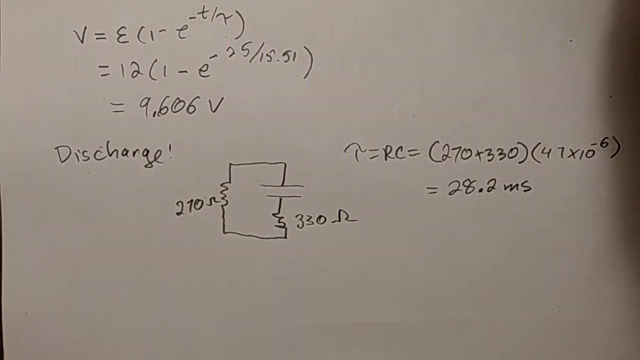 Hmm, I'm just you know what. Oh, there's my calculator. I realized that in my prepared notes I didn't do it that way, And that's kind of silly. If we want the potential across a resistor, the best thing to do is to get the current through the resistor. So what I'm going to do, 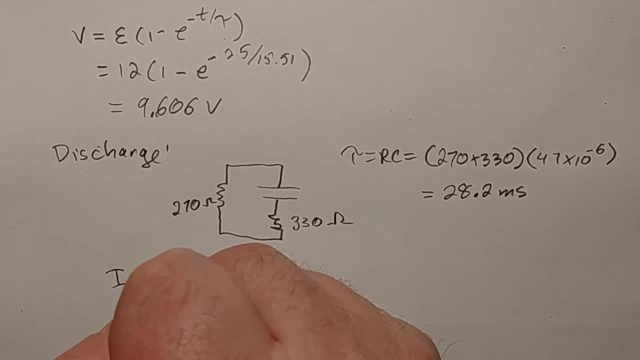 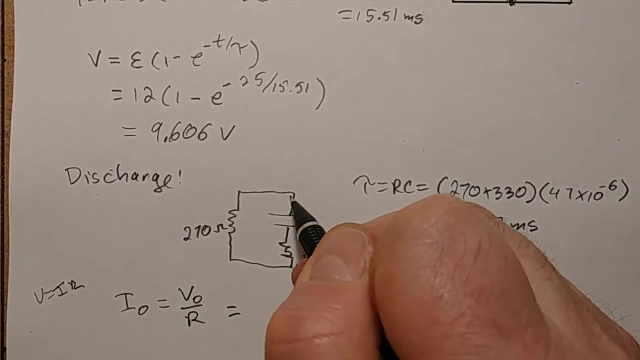 is. I'm going to find out what is the potential across the resistor And I'm going to find out what is. I naught Remember, V equals IR. So I naught equals V, naught over R. So the initial voltage, it says, was the voltage that we had. This was at 9.606 volts. That was what was forcing. 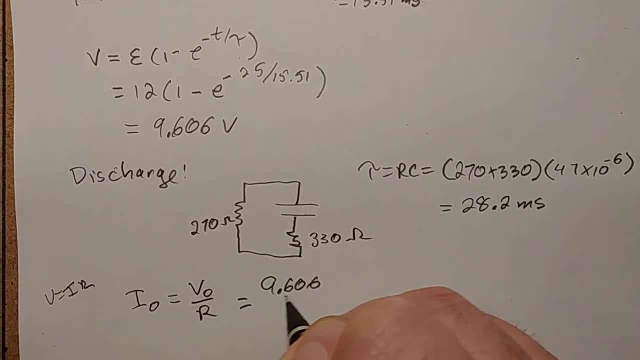 charges through the resistors: 9.606.. And we're going to divide that by the total resistance, which is 270 plus 330, which is 600.. So 9.606 divided by 600 is 0.01601.. 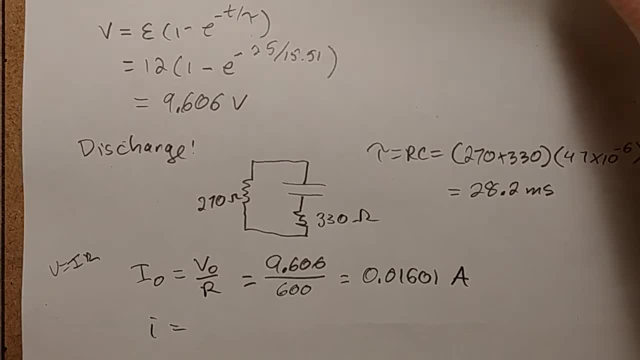 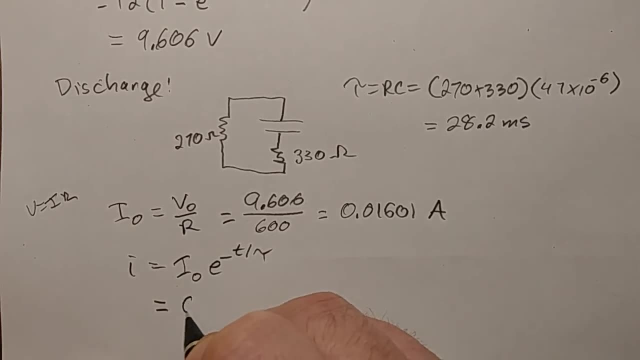 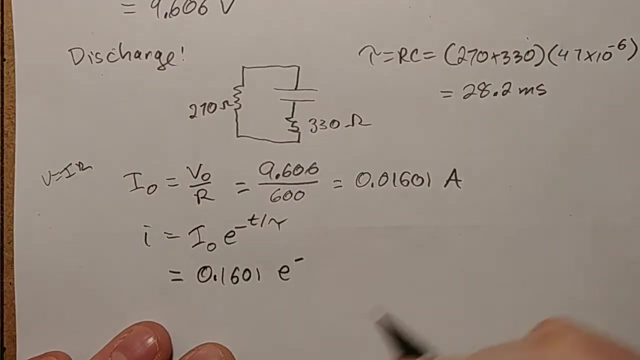 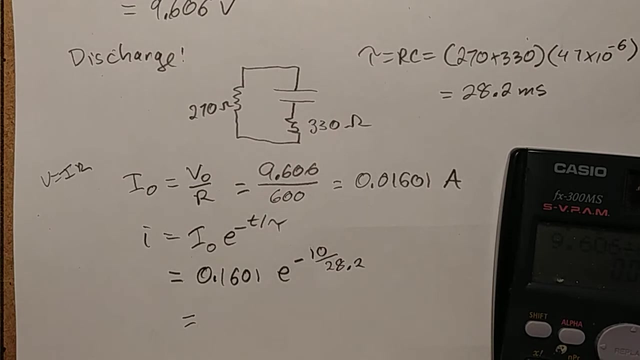 That is. I naught, Well, I equals. I naught E to the negative, T over tau, So that's equal to 0.1601 E to the negative. And it said 10 milliseconds after the switch is opened. So negative 10 over 28.2 equals. what do I get? 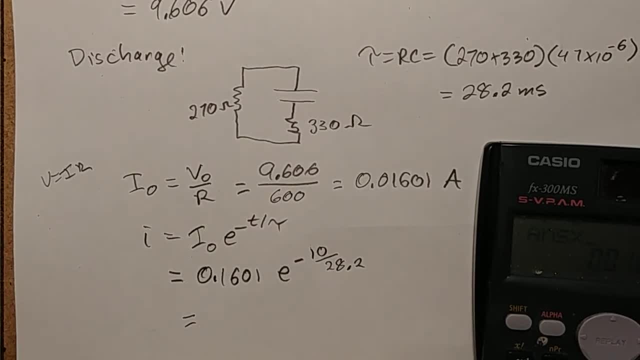 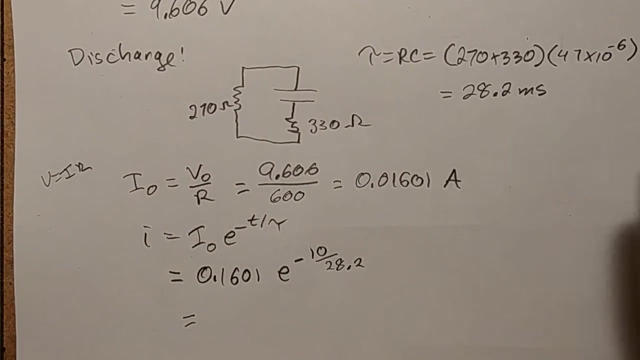 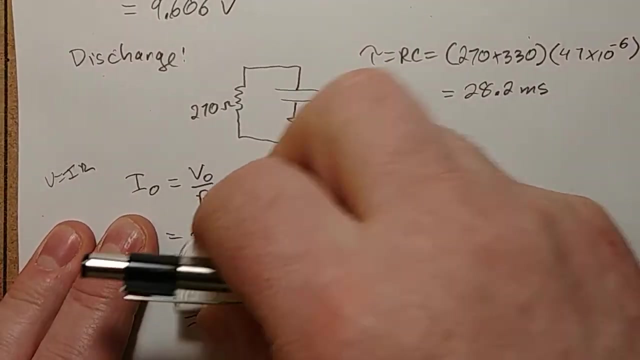 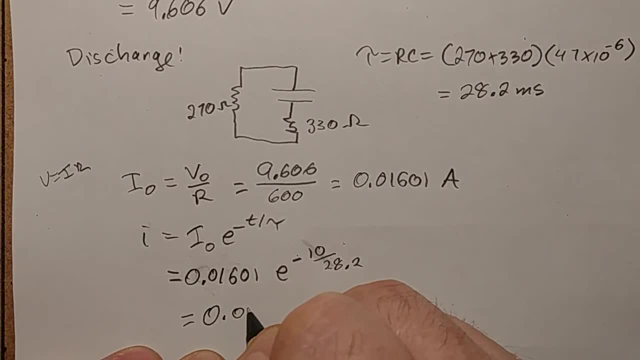 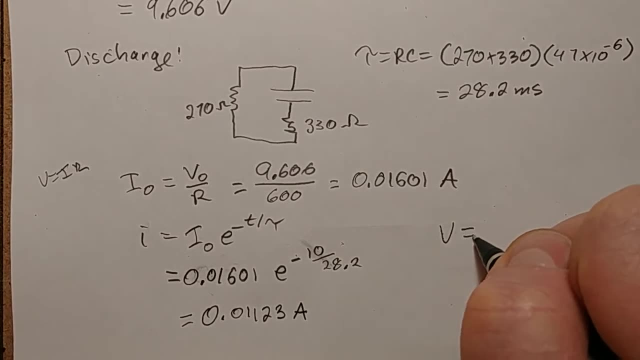 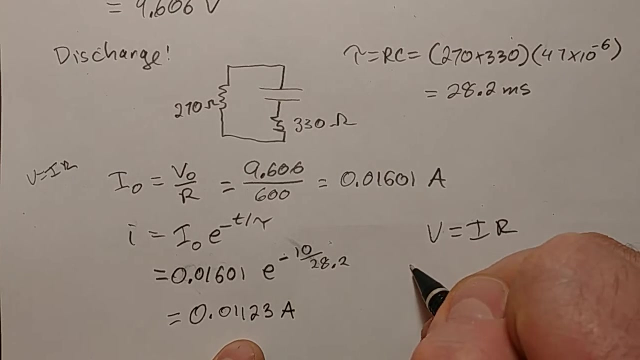 0.01223.. 1123.. But V equals IR And we want to know the voltage now, just across the 270 ohm resistor. So what we have is we have 0.116.. Now there's only 1.235.. 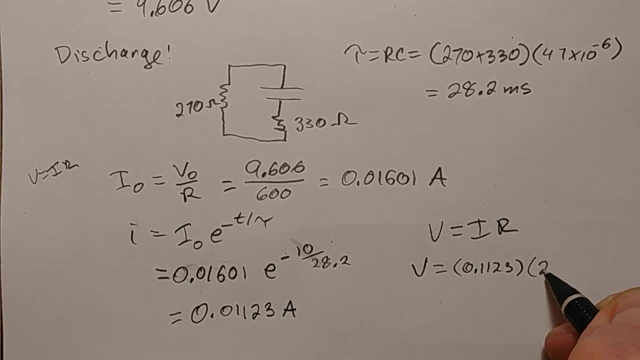 So we're going to take the 3.023 amps going through that resistor, And just that resistor itself has 270 ohms of resistance. So if we multiply this times 270, we get 3.03 volts. So there you go.